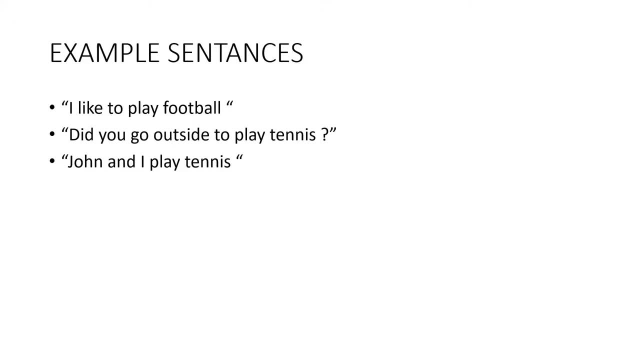 Friends, welcome to my channel, Dhanesh here. In this video we will implement the TF-IDF scheme from scratch in Python. The term TF stands for term frequency, while the term IDF stands for the inverse document frequency. What are the problems with the Bag of Words model? 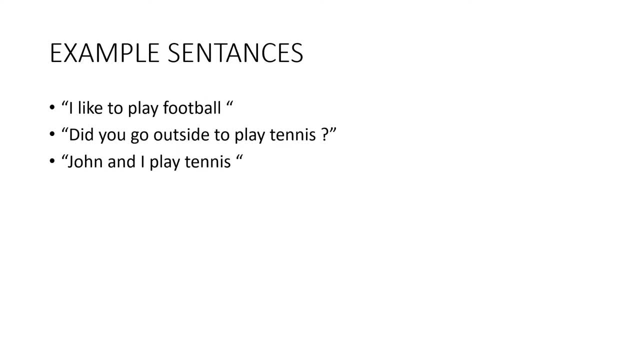 Before we actually see the TF-IDF model, let us first discuss a few problems associated with the Bag of Words model. We have the following three example sentences: I like to play football- Did you go outside, John? and I play tennis. The resulting Bag of Words model looks like this: 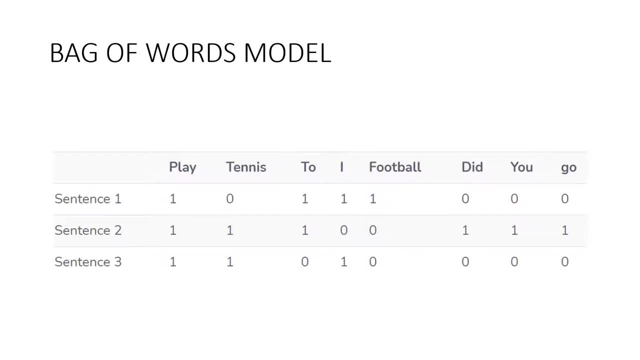 One of the main problems associated with the Bag of Words model is that it assigns equal values to the words, irrespective of their importance. For example, the word play appears in all the three sentences. Therefore, this word is very common. On the other hand, the word football only appears in one sentence. 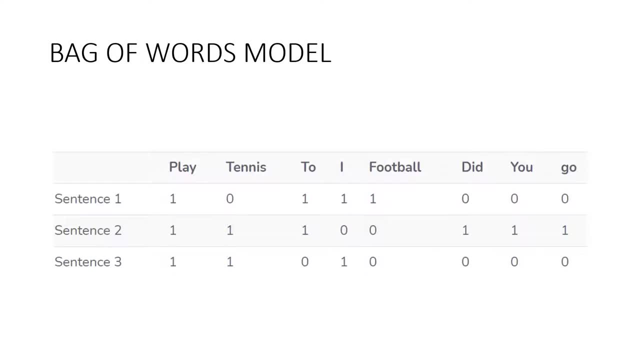 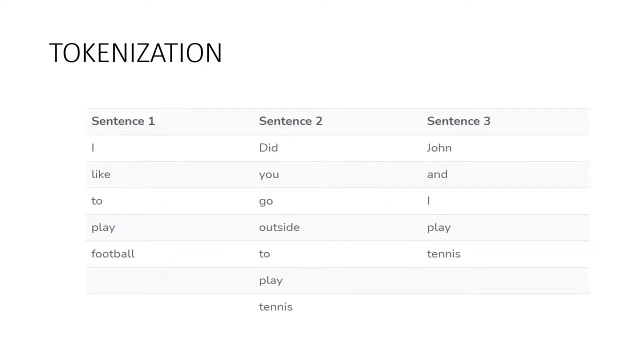 The words that are played only with the bag and not other- with the bag rare- have more classifying power compared to the words that are common. The idea behind the TF-IDF approach is that the words that are common in one sentence and less common in the other sentence should be given high weights. 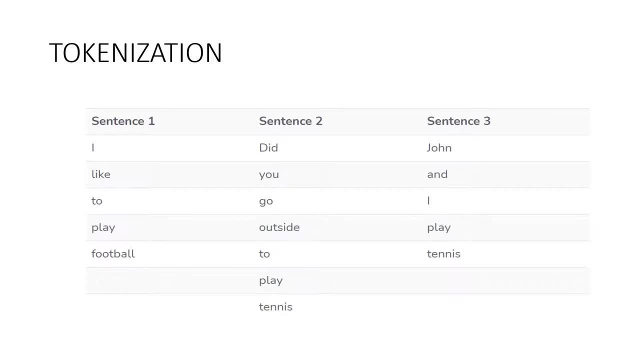 Before implementing the TF-IDF scheme in Python, let's first understand the theory. We will use the same three sentences as our example as we used in the bag of words model. – I like to play football. did you go outside to play tennis, John and I play tennis. 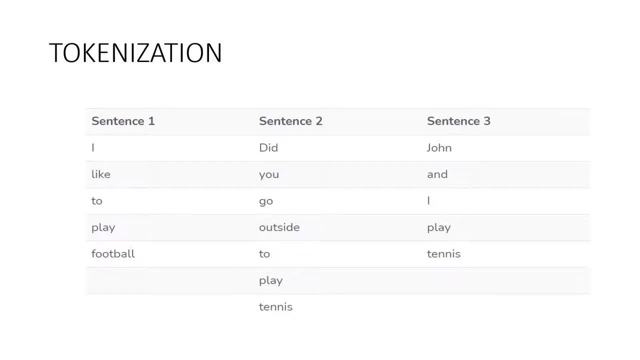 Step 1 is the tokenization. Like the bag of words, the first step to implement the TF-IDF model is tokenization. You can see here: sentence 1, sentence 2 and sentence 3 is tokenized. Step 2 is to find the TF-IDF values. 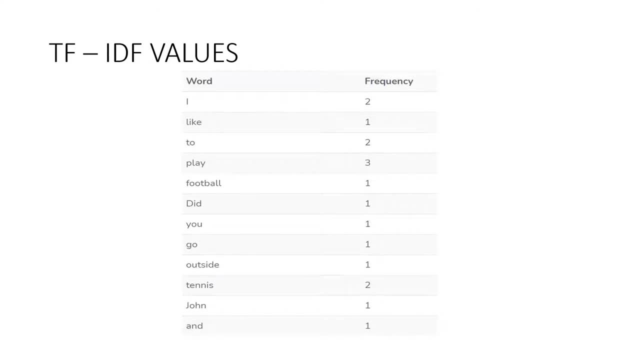 Once you have tokenized the sentences, the next step is to find the TF-IDF values. You will see here that the TF-IDF values are called the terms. Step 2-2 are the slapping terms. We are going to use the TF-IDF values for each word in the sentence. 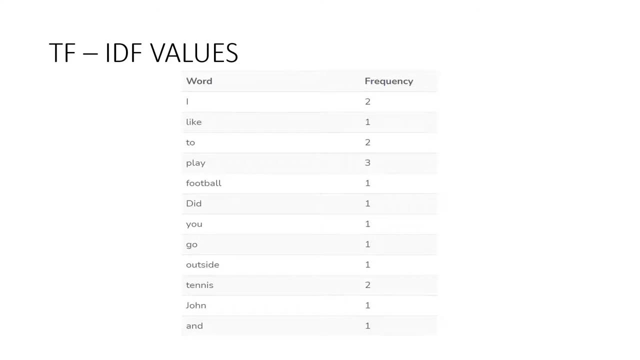 As discussed, the TF-IDF values refer to the term frequency and can be calculated. TAFR can be calculated using test test response. You may add TIFF values. � rectangular, pariat, simultaneous, reticulous, tri ankles. trip 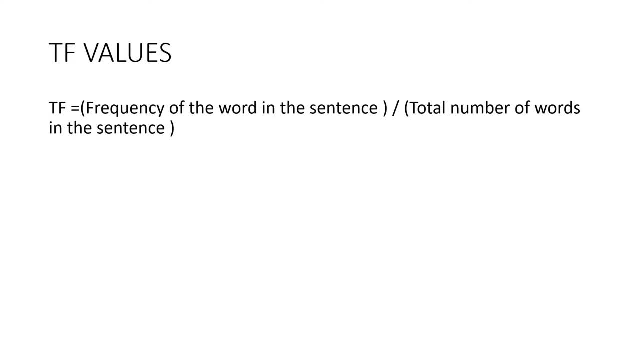 rtf is equal to frequency of the word in the sentence divided by total number of words in the sentence. for, for instance, uh, look at the word play in the first sentence, its term frequency will be 0.20, since the word play occurs only once in the sentence and the total number of words in the 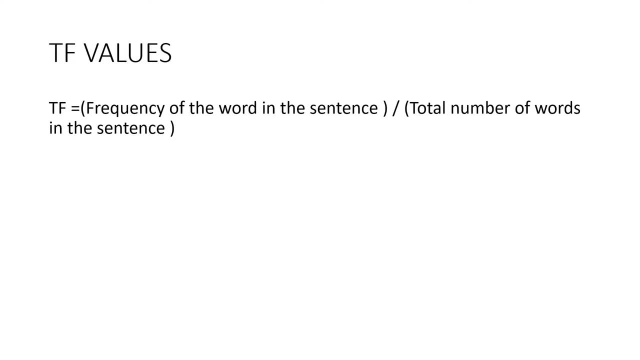 sentence are 5, hence 1 by 5 it is 0.20. idf refers to the inverse document frequency and can be calculated as follows: idf is equal to total number of sentences, that is, documents divided by number of sentences, that is, documents containing the word. 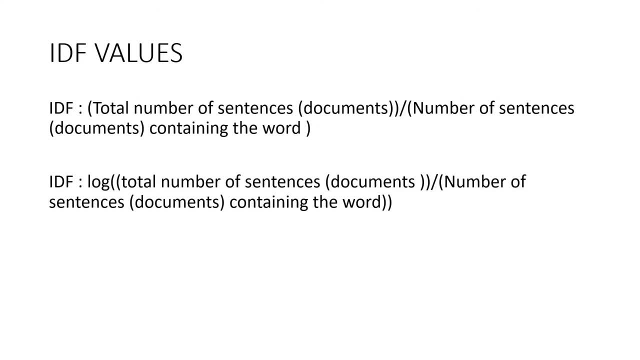 it is important to mention that the idf values for a word remains the same throughout all the documents and it depends upon the total number of documents. on the other hand, tf values of a word differ from document to document. let us find the idea frequency of the word play, since we have 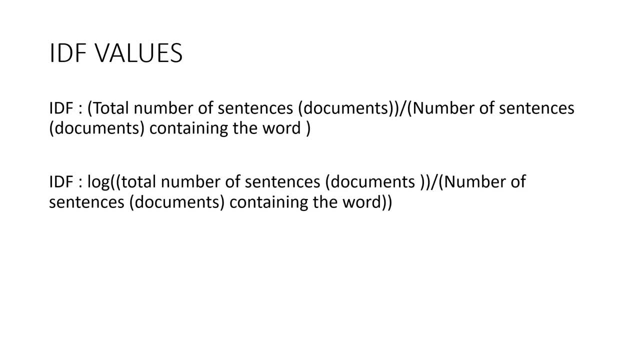 three documents and the word play occurs in all three of them. Therefore, IDF value of the word play is 3 by 3, equal to 1.. TF-IDF values are calculated by multiplying TF values with their corresponding IDF values. To find the TF-IDF value, we first need to 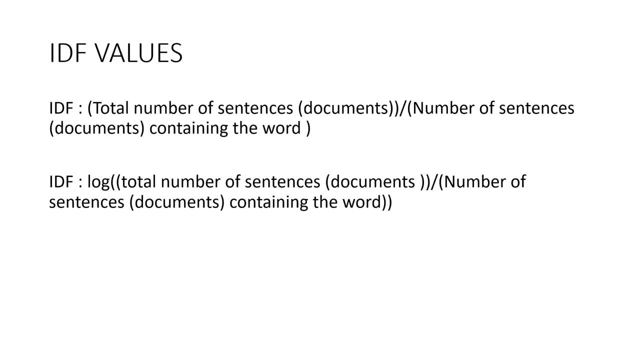 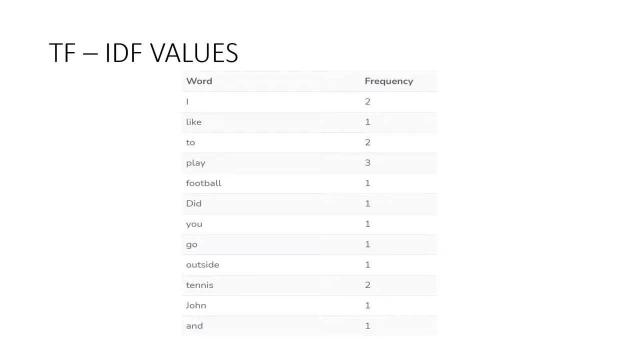 create a dictionary of word frequencies, as shown here. This is the word frequency. You can see word i, frequency 2, like it's 1.. So let's sort the dictionary in the descending order of the frequency It's shown here. Now we will filter the 8 most frequently occurring words. 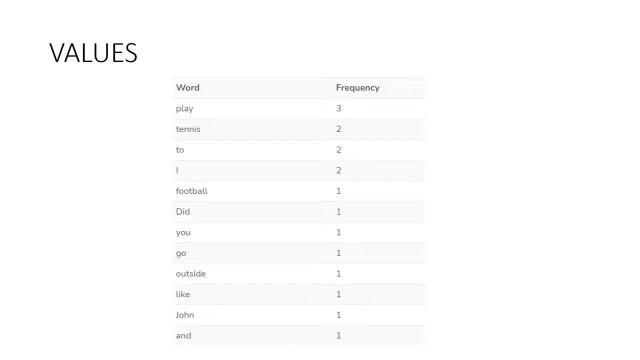 As I said earlier, since IDF values are calculated using the whole corpus, we can calculate the IDF values for each word. now The next table contains IDF values For each table. this is the IDF values. You can clearly see that the words that are rare have higher IDF values compared to the 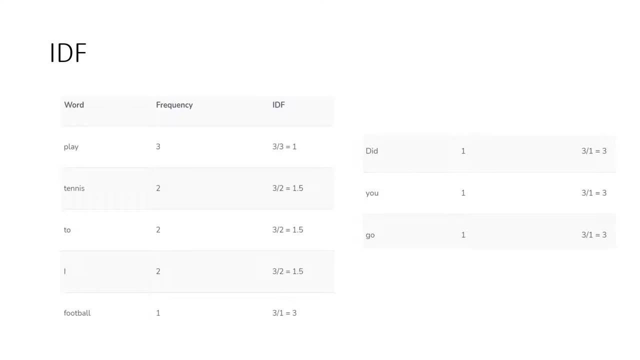 words that are more common. Let's now find the TF-IDF values for all the words in each sentence. Let's find the TF-IDF values for all the words in each sentence. Let's find the TF-IDF values for all the words in each sentence. 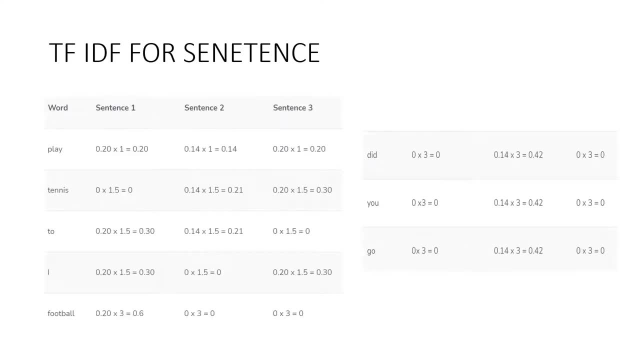 The values in the columns for sentences 1,, 2 and 3 are corresponding TF-IDF vectors for each word in the respective sentences. The values in the columns for sentences 1, 2 and 3 are corresponding TF-IDF vectors for. 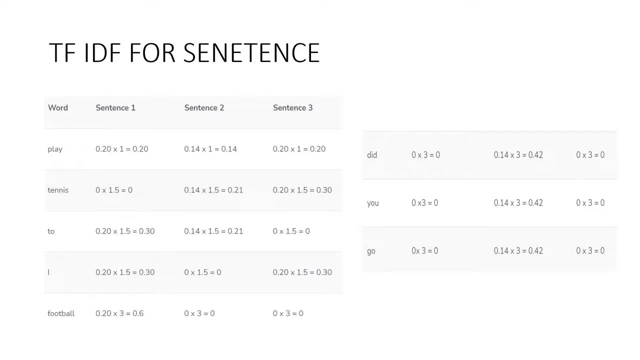 each word in the respective sentences. The values in the columns for sentences 1, 2 and 3 are corresponding TF-IDF vectors for each word in the respective sentences. The values in the columns for sentences 1, 2 and 3 are corresponding TF-IDF vectors for. 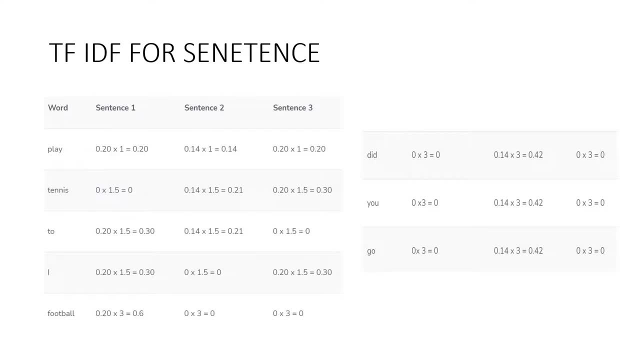 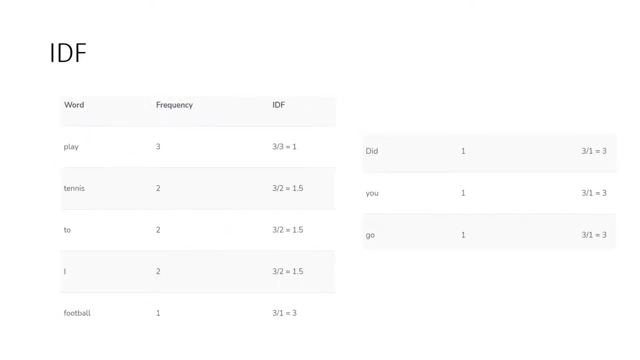 each word in the respective sentences. As you can see, we can calculate the log of the IDF values using IDF values to mitigate the effects of very rare and very common words on the corpus, before multiplying it with TF-IDF value. In such case, the formula for IDF will be this: 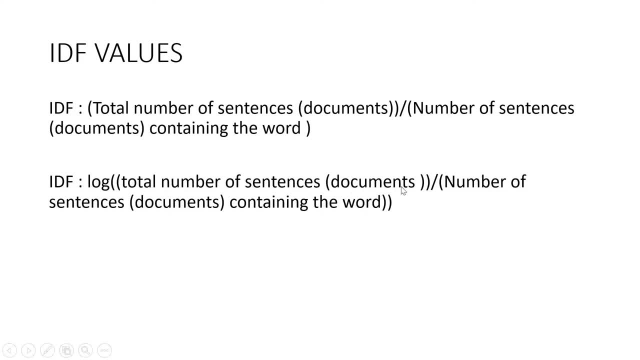 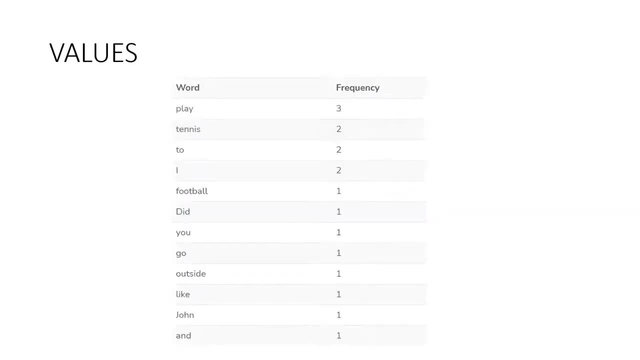 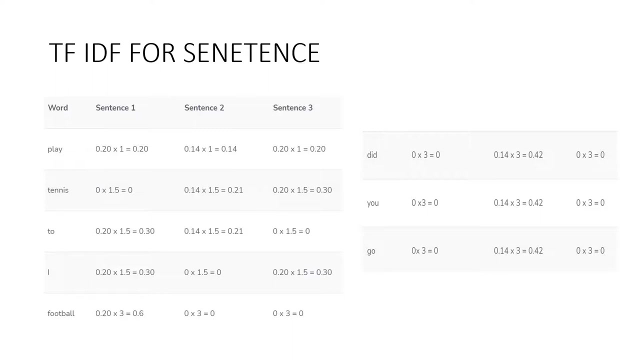 IDF will be log: total number of sentences. document: Document sentence divided by number of sentence documents containing the word. We need to take the log of the previous this one. So since we had only three sentences in the corpus, for the sake of simplicity we did. 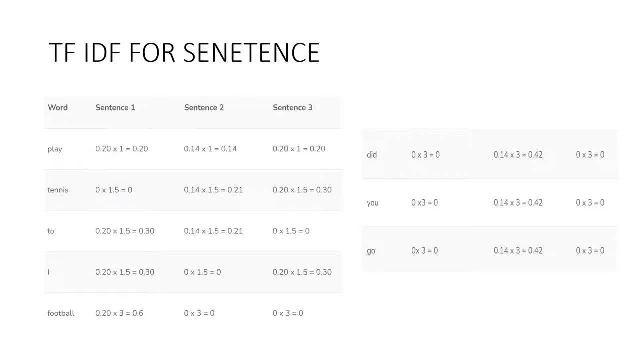 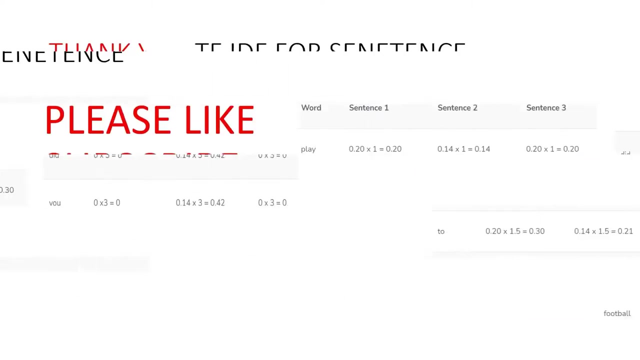 not use the log In the implementation section. we will use the log function to calculate the final TF-IDF values In this table. we didn't use See. let's do the TF-IDF model from scratch in Python, As explained. 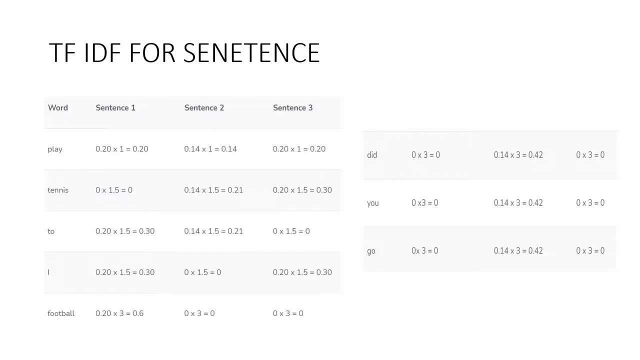 In theory, the steps to create a sorted dictionary of word frequency is similar between the Bag of words model and TF-IDF model. To understand how we create a sorted dictionary of word frequencies, I will explain. TF-IDF model will be built upon a Python library. 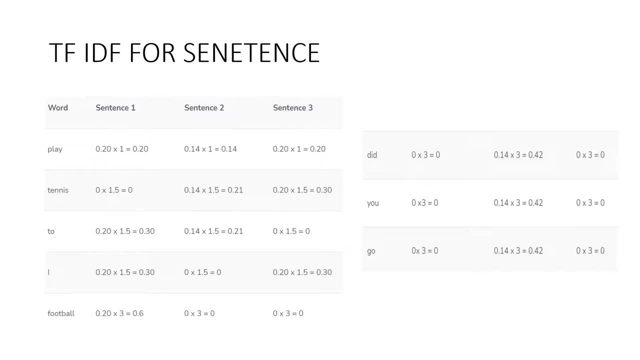 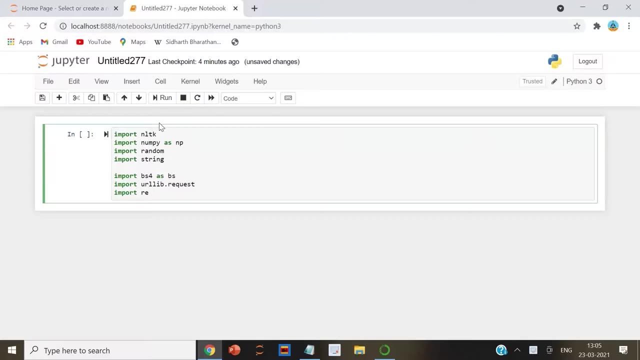 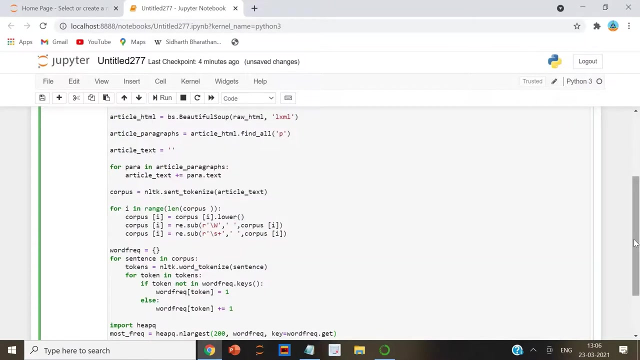 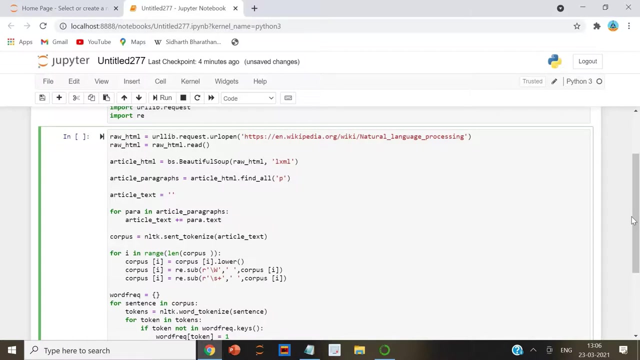 and I will be using NLTK NumPy. These are all the libraries I am using. I have just imported the necessary libraries. So if you see this script, I have written the script here In the script. we first grabbed the Wikipedia article on. 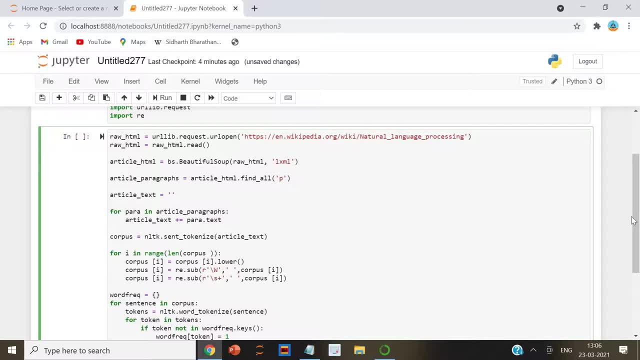 natural language processing. We then pre-processed it to remove all the special characters and multiple empty spaces. Finally, we create a dictionary of word frequencies and then filter the top 200 most frequently occurring words. The next step is to find the IDFS values for the most frequently occurring words in the corpus. Let me do. 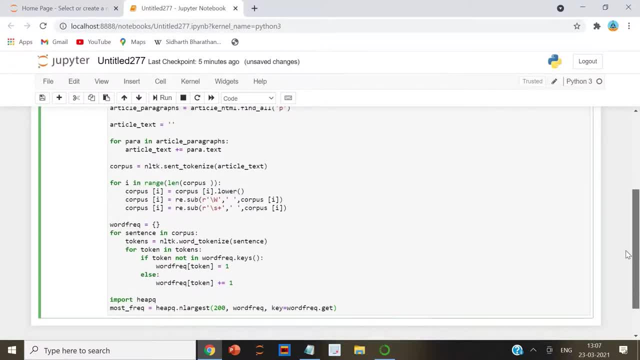 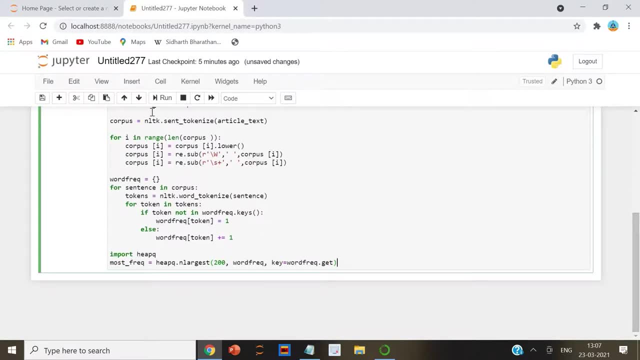 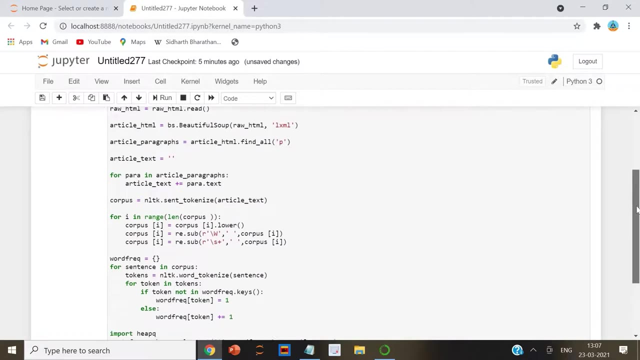 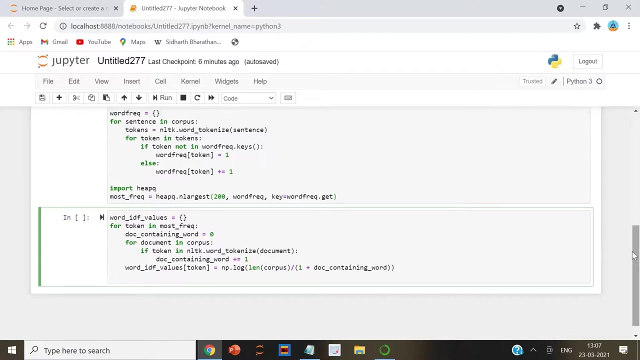 this. First let me run this. In this script I create an empty dictionary- word__IDFValues. This dictionary will store most frequently occurring words as keys and their corresponding IDF values as dictionary values. Next we iterate through the list of most frequently occurring words. 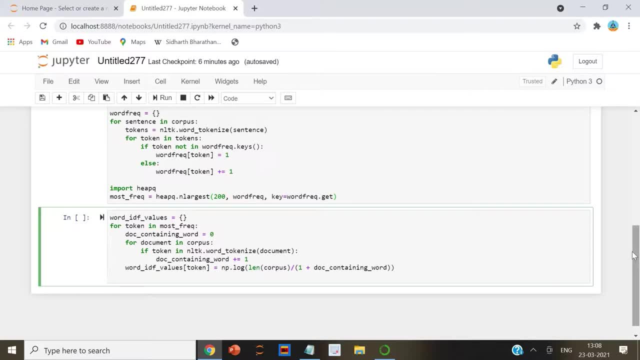 During each iteration we create a variable doc containing word. This variable will store the number of documents in which the word appears. Next we iterate through all the sentences in our corpus. The sentence is tokenized and then we check if the word exists in the sentence or not. 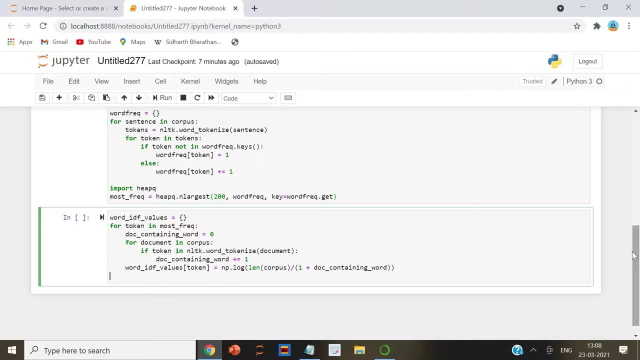 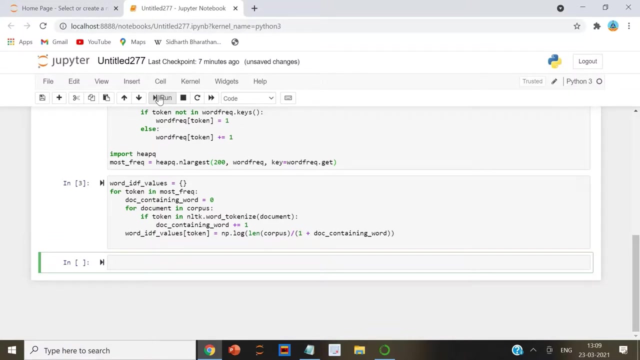 If the word exists, we implement the doc containing word variable. Finally, to calculate the IDF value, we divide the total number of sentences by the total number of documents containing the word. The next step is to create the tf dictionary. for each word In the tf dictionary, the key 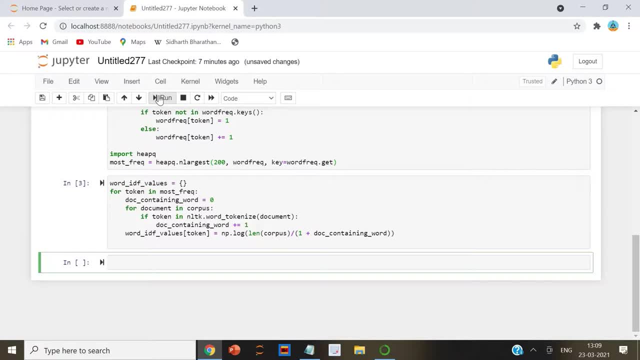 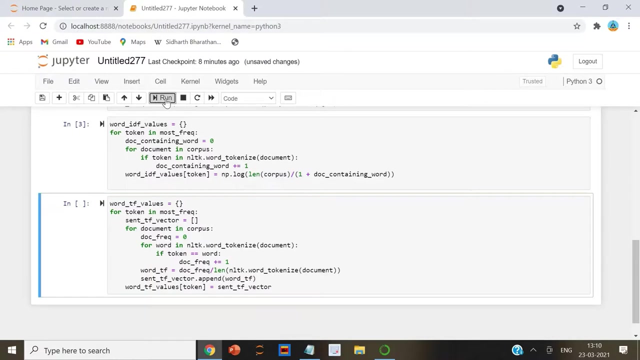 will be the most frequently occurring words, while the values will be 49-dimensional vectors. Since our document has 49 sentences, each value in the vector will belong to the tf values of the word for the corresponding sentence. Let me run this. Yeah, it's working. 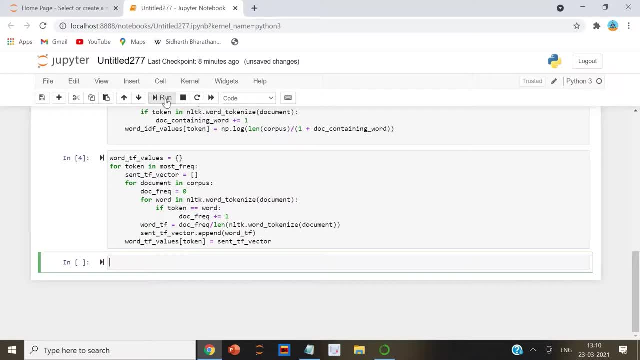 So in this script we create a dictionary that contains the word as the key and the list of 49 items as the value, since we have 49 sentences. We then iterate through all the sentences in the corpus as discussed. Each item in the list stores the tf value of the word for the corresponding sentence. 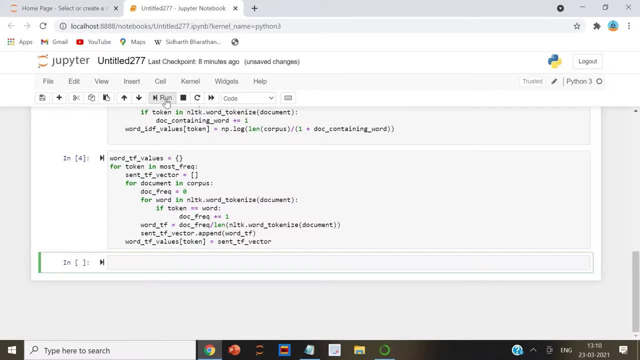 In the script above. word underscore- tf, underscore values is our dictionary. For each word we create a list sentence underscore- tf- underscore vector. We then iterate through each sentence in the corpus and tokenize the sentence. The word from the outer loop is matched with each word in the sentence, So the word is the only one in the. 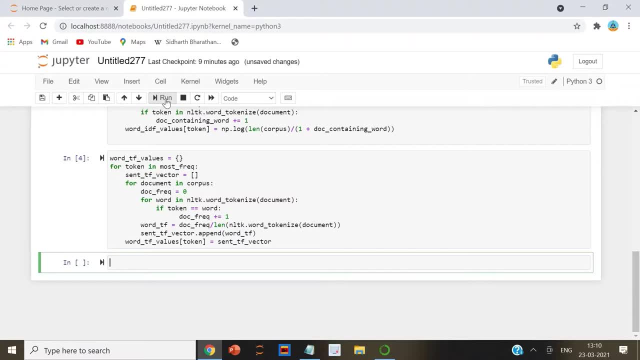 word in the sentence. If a math is found, the doc-frequency variable is incremented by one. Once all the words in the sentence are iterated, the doc-frequency is divided by the total length of the sentence to find the tf value of the word for that sentence. 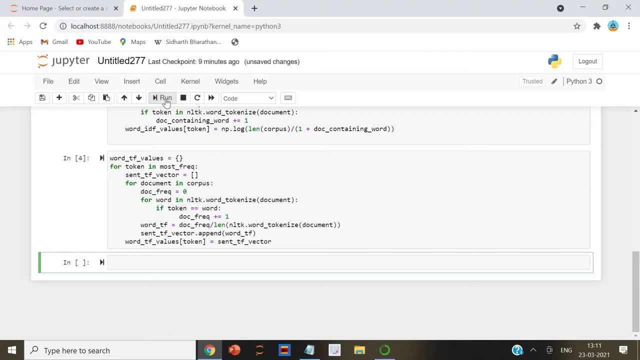 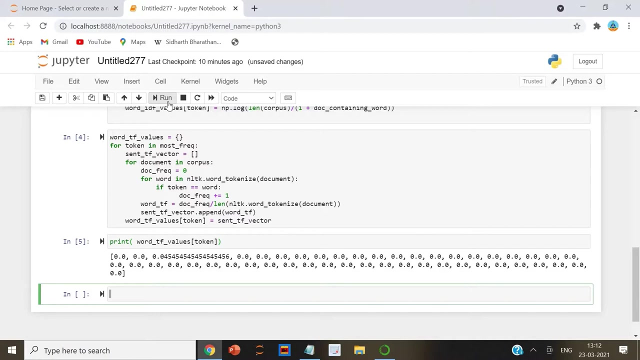 This process repeats for all the words in the most frequently occurring word list. The final word-tf-values dictionary will contain 200 words as keys. For each word, there will be a list of 49 items as the value. Now we have idf values of all the words along with tf values for every word across the sentences. 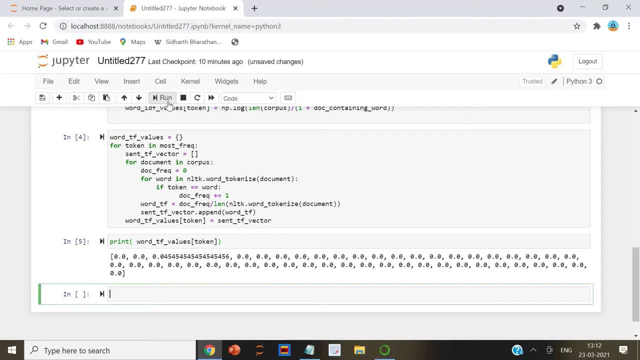 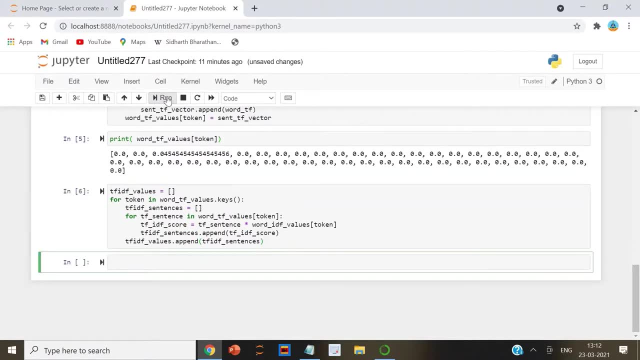 The next step is to simply multiply idf values with tf values. In this script we create a list called tfidf- underscore values. We then iterate it through the idf values. All the keys in the word underscore: tf, underscore values- dictionary. These keys are basically the most frequently occurring words. 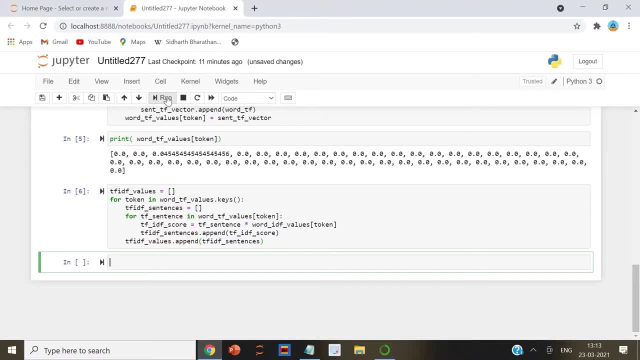 Using these words, we retrieve the 49-dimensional list that contains the tf values for the word corresponding to each sentence. Next, the tf value is multiplied by the idf value of the word and stored in the tf underscore. idf underscore score variable.